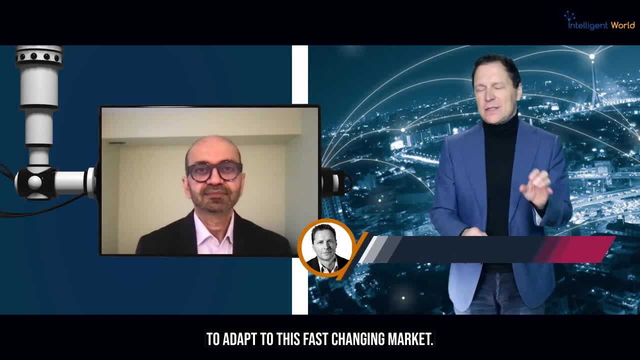 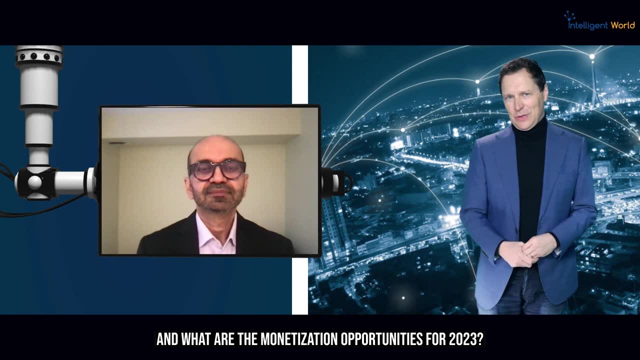 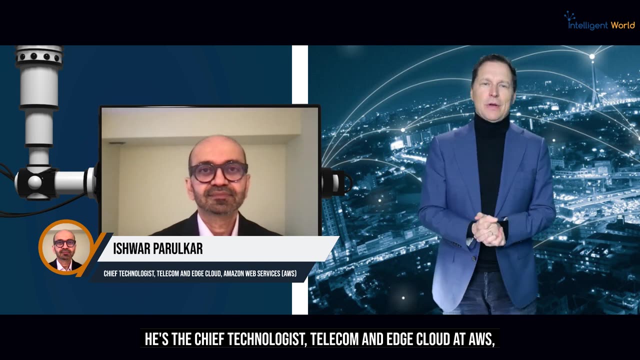 The telecom industry is always under pressure to adapt to this fast-changing market. What are the key areas of new tech development and what are the monetization opportunities for 2023?? Today we have Ishwar Parulkar. He is the Chief Technologist, Telecom and Edge Cloud at AWS. 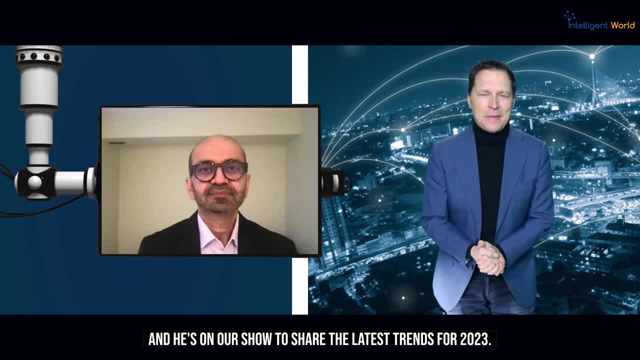 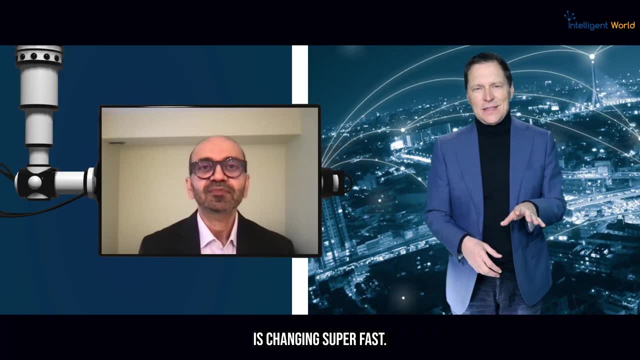 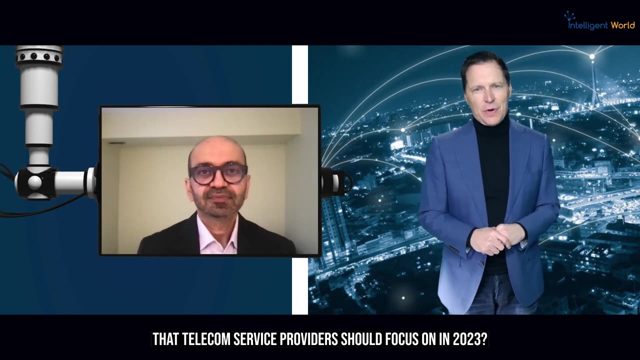 And he's on our show to share the latest trends for 2023.. Welcome, Ishwar. Happy to be here. Ronald, As mentioned, the telecom industry is changing super fast. What are the top digital transformation priorities that you see, And what are areas that telecom service providers should focus on in 2023?? 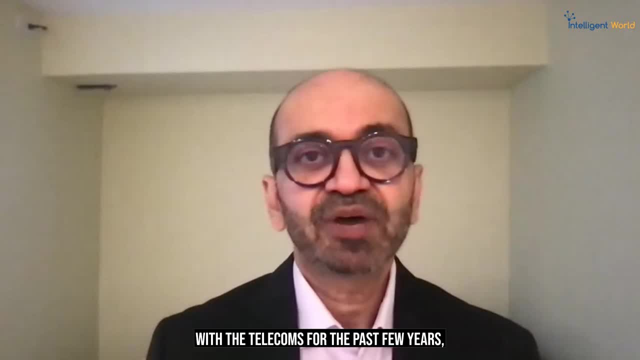 So at AWS, we've been working with telecoms for the past few years, But we really believe that 2023 is going to be an inflection point And we're going to see acceleration in some areas and some new focus areas pop up. 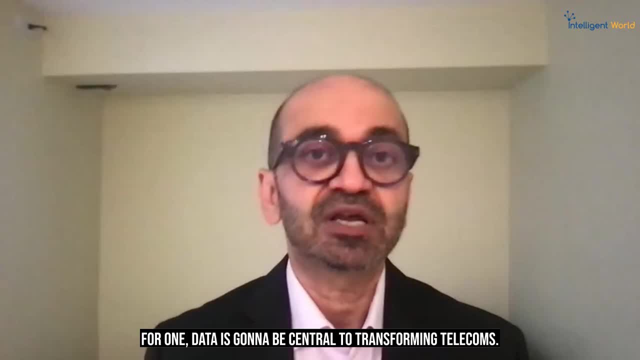 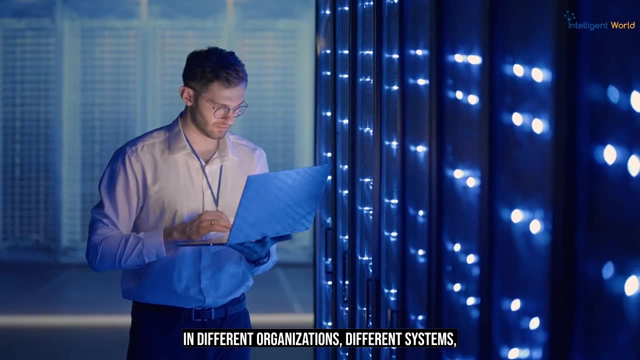 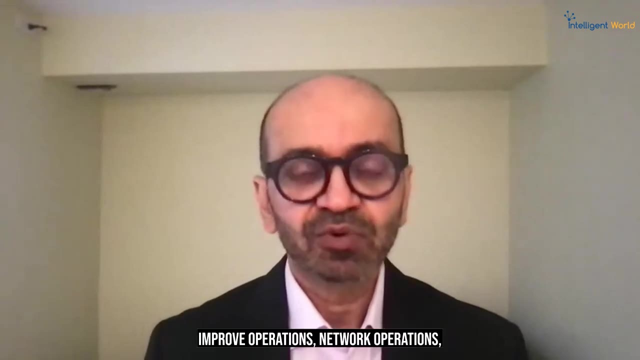 For one data is going to be central to transforming telecoms. Telcos have a lot of data Today, but it's in silos sitting in different organizations, different systems, And there's a lot of potential in really harnessing this data to not only improve operations, network operations. 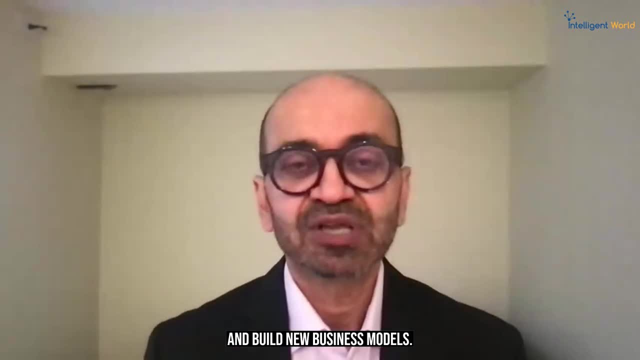 but also really change the customer experience and build new business models. So we'll see a fair bit of that happening with third-party cookies. depreciating First-party data becomes super important And obviously this has to be done with customers' best interest. 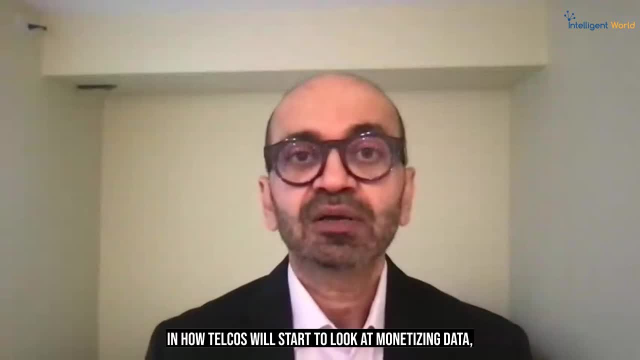 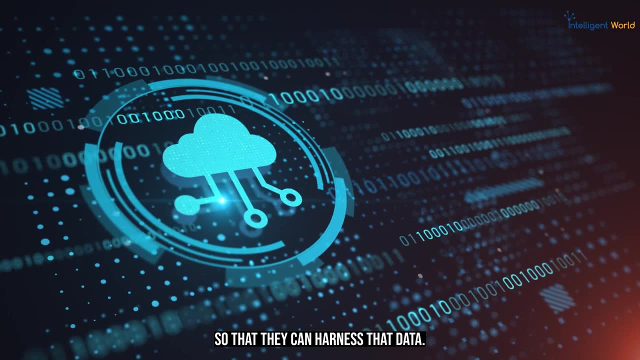 But that's going to be another change in how technology telecoms will start to look at monetizing data and then you know kind of modernizing the data infrastructure using the cloud so that they can harness that data. So that's number one. 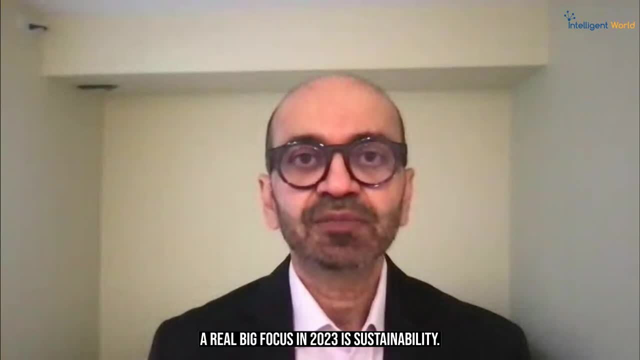 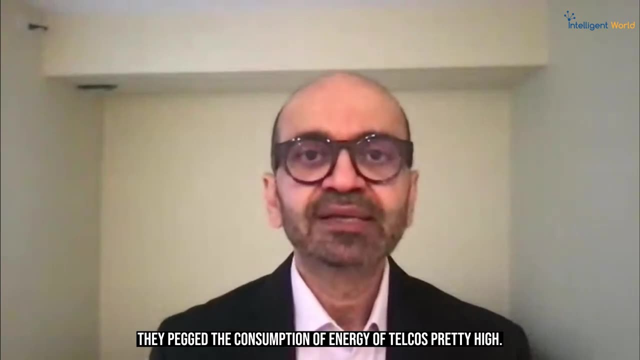 The second area where we would see a real big focus in 2023 is sustainability. If you look at various research reports, they peg the consumption of energy of telcos pretty high. The carbon dioxide emissions of telcos are approximately 3%. So if you look at the carbon dioxide emissions of telcos, 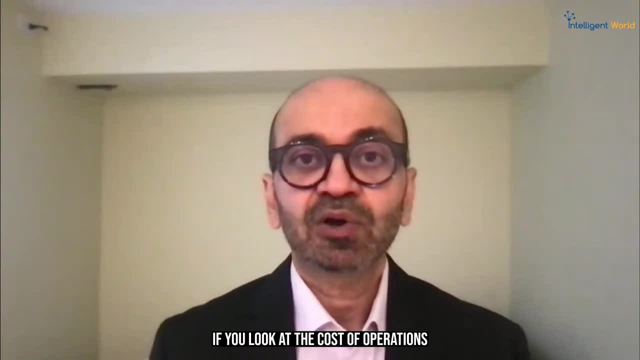 you can see that the carbon dioxide emissions of telcos are approximately 3% to 4%, which is twice that of the aviation industry, which is heavily scrutinized in this space. If you look at the cost of operations attributed to energy consumption. 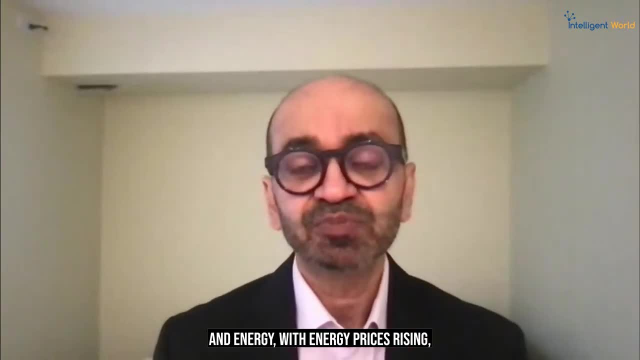 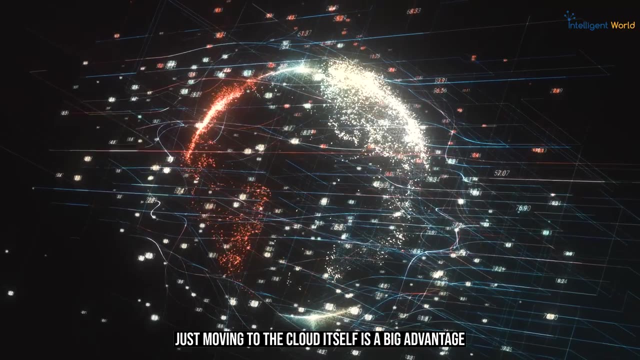 it's anywhere between 15% to 40%, you know, according to various research reports. So it is a big problem for them. and energy- with energy prices rising, it becomes even more critical. Here also, the cloud is a big enabler. 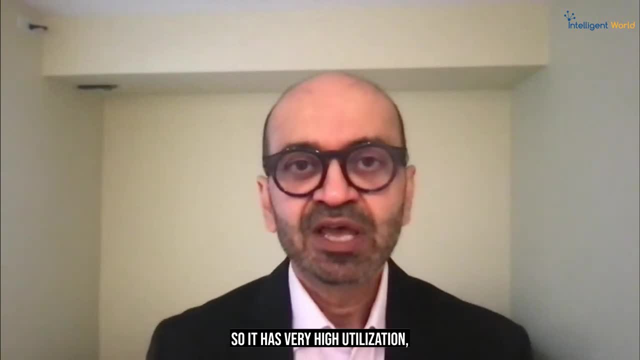 Just moving to the cloud itself is a big advantage because cloud is large scale, multi-tenant, so it has very high utilization And research 451 has shown that just moving to the cloud improves carbon footprint by 80%. And at MLS we are focused on renewable energy. 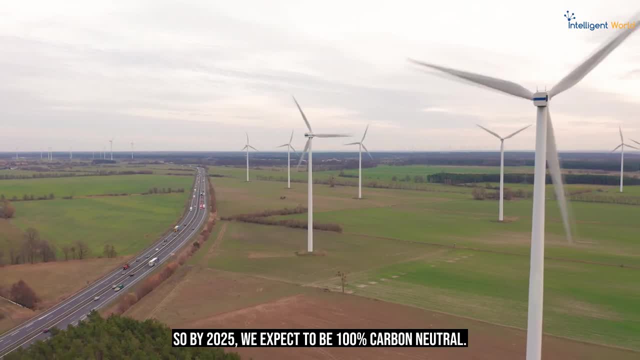 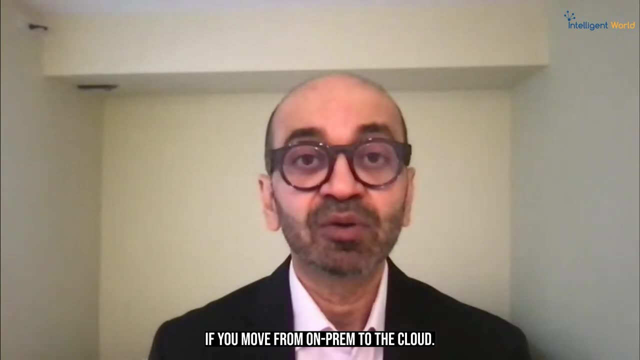 So by 2025, we expect to be 100% carbon neutral. With that, this carbon footprint from 80% goes to a 90% improvement if you move from on-prem to the cloud. So just by moving to the cloud itself. 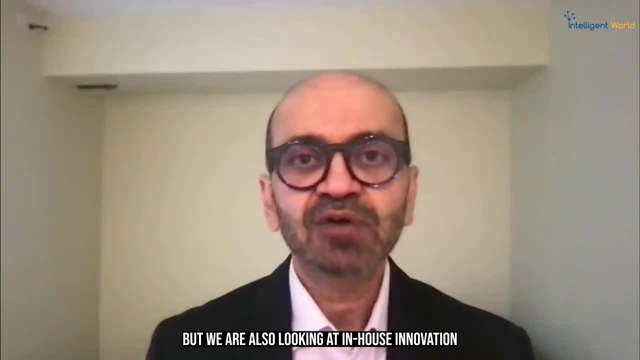 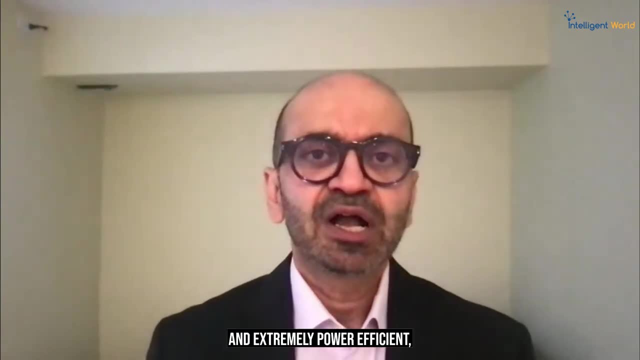 telcos can benefit from it, But we are also looking at in-house innovation, like using Graviton processors, which are ARM-based processors and extremely power efficient, And we are seeing improvement in telco workloads. 5G packet core. 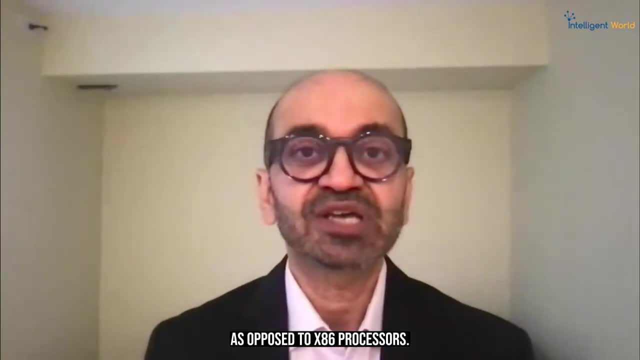 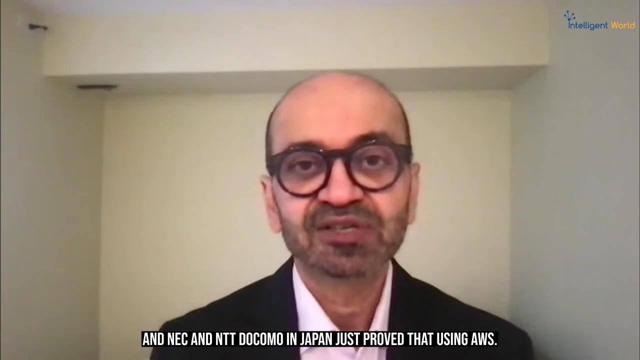 of up to 70% in using these processors as opposed to x86 processors, And NEC and NTT DoCoMo in Japan just proved that using AWS. So that was the second transformation I see, which is sustainability- It's becoming very focused and cloud being an enabler. 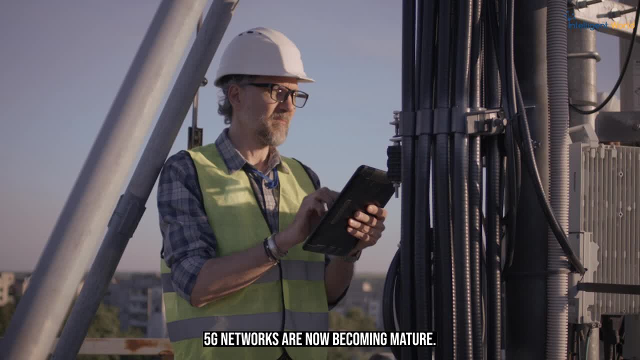 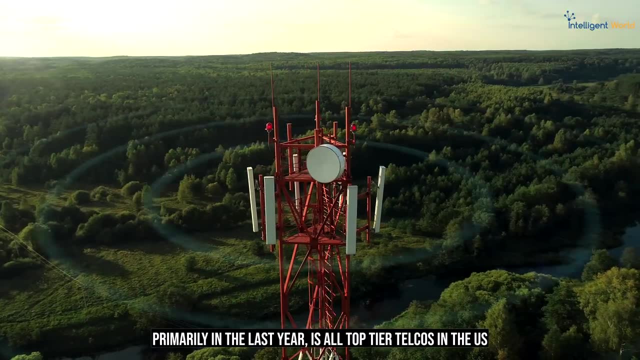 The third one is around really monetizing 5G. 5G networks are now becoming mature. If you look at what has happened until now, primarily in the last year, is all top-tier telcos in the US now have 5G networks. 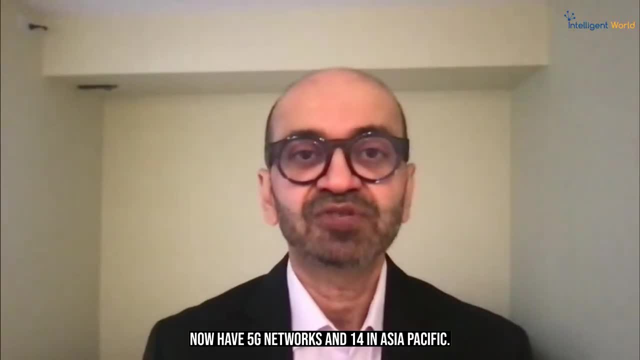 34 of the 50 countries in Europe now have 5G networks and 14 in Asia Pacific. So now there's an entrenched footprint of 5G. We'll see the next level of really adopting 5G and unleashing the power of 5G, which it was intended to be. 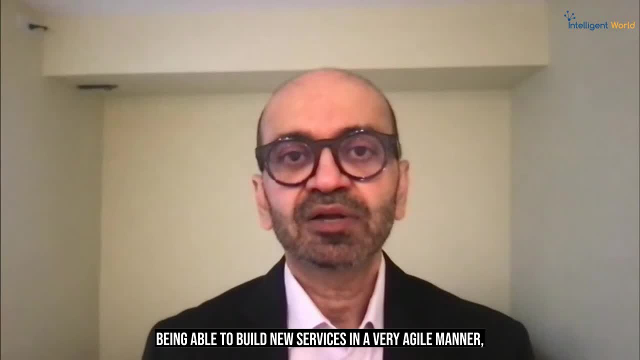 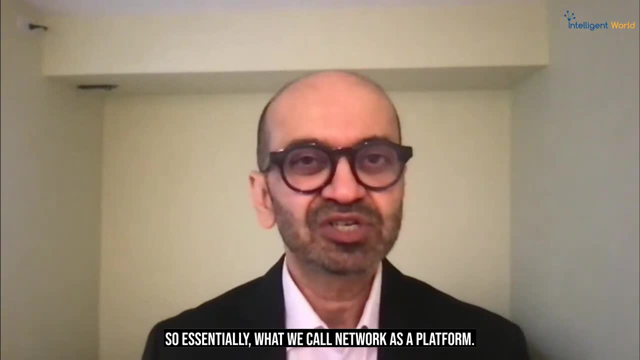 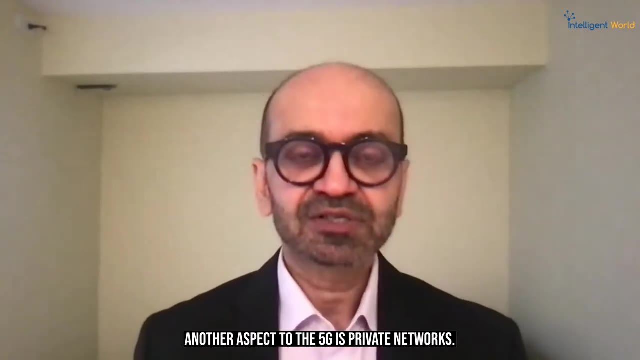 Very dynamic networks, being able to build new services in a very agile manner, personalizing the services based on customers, and so forth. So essentially what we call network as a platform. We'll see more of that happening. Another aspect to the 5G is private networks. 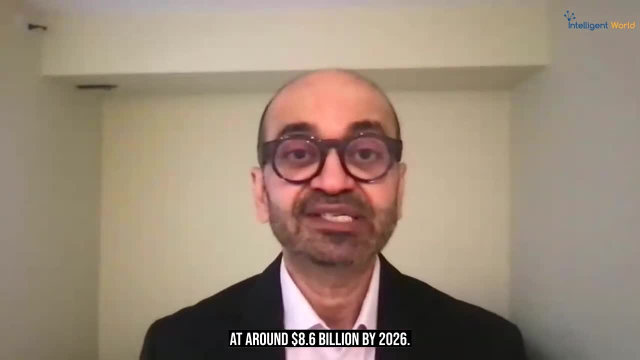 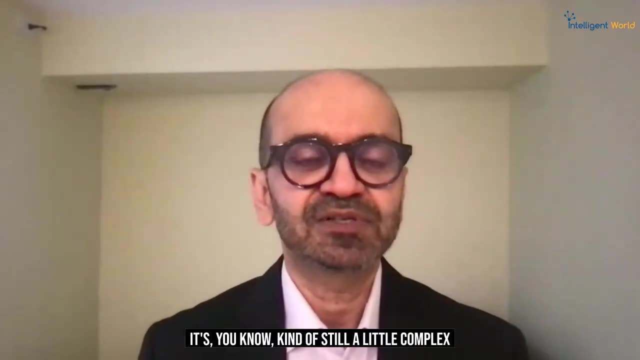 IDC research has pegged the market at around $8.6 billion by 2026.. Now, admittedly, the 5G network is not the only one. The adoption has been slow because of various challenges. It's, you know, kind of still a little complex to set them up. 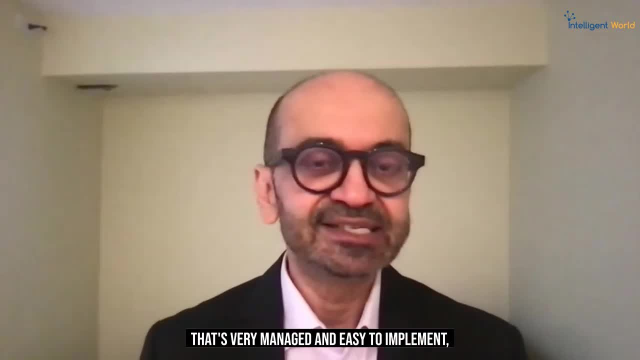 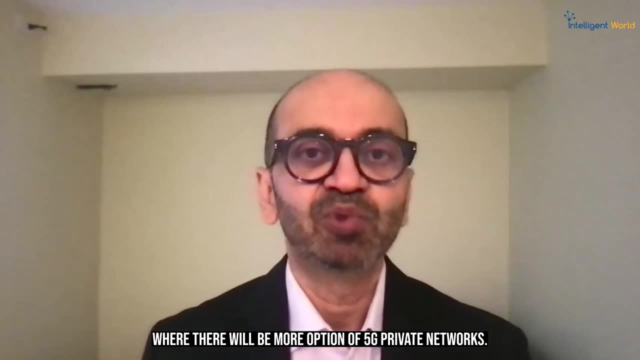 So you need an experience that's very managed and easy to implement, which is what we've been focused on on AWS. But in 2023, we'll see an inflection point where there will be more adoption of 5G private networks. 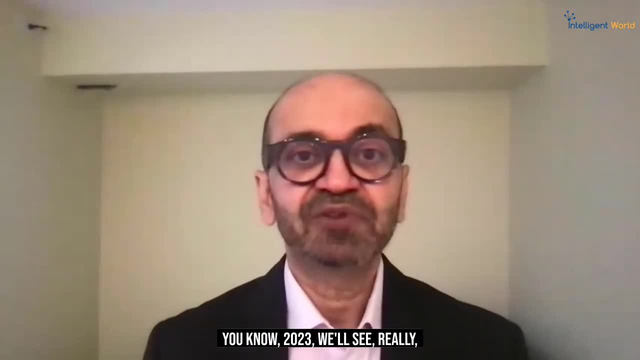 So that was point number three, which is, you know, 2023, we'll see really telcos starting to monetize 5G. And the last point where I see the focus in 2023, is telcos trying to become techcos. 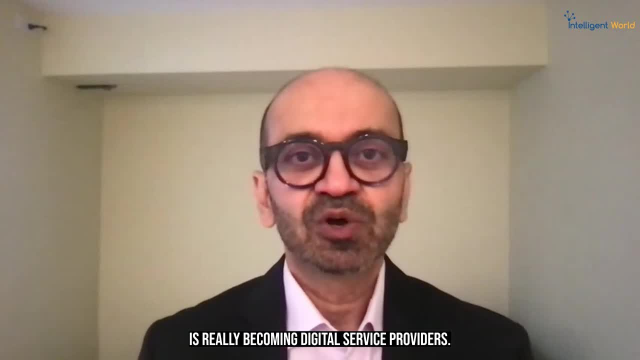 What I mean by that is really becoming digital service providers. So, instead of just providing connectivity, providing services like training and staffing to enable their customers to move to the cloud. So we have actual telco partners working on programs like this, like Swisscom. 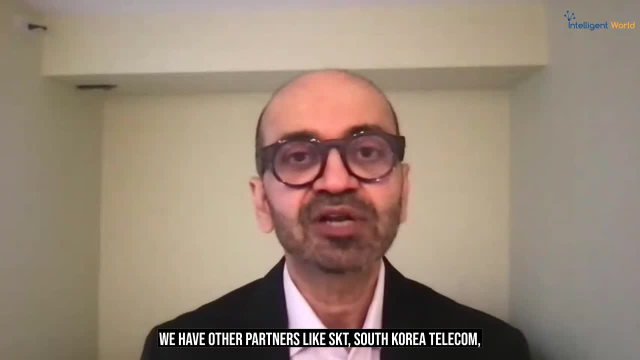 We have other partners like SKT, South Korea Telecom, working on becoming an AI-oriented company and developing services which have a lot of AI technology in them. So this is the fourth pillar, I think, of what I see as a transformational opportunity for telcos in 2023,. 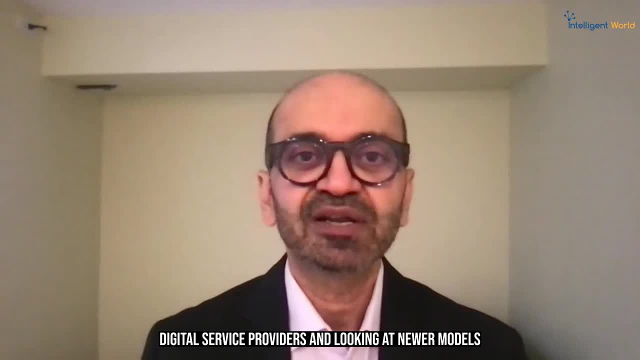 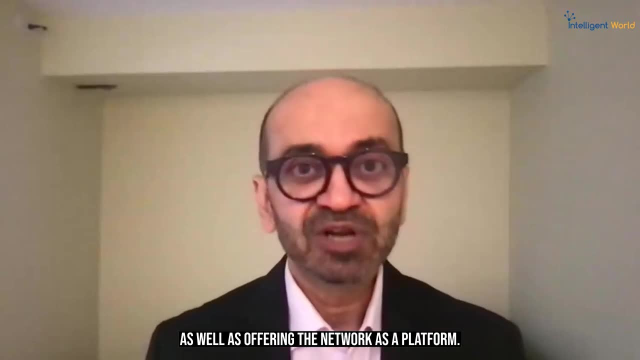 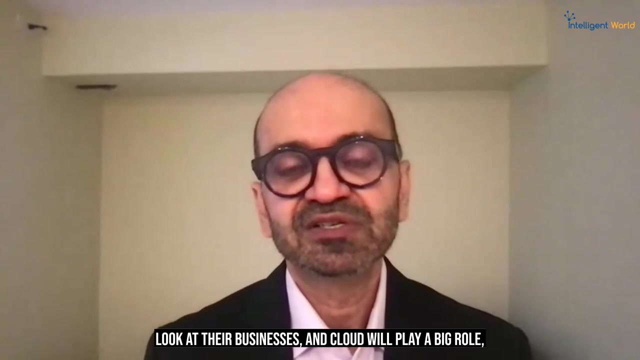 which is starting to really becoming digital service providers and looking at newer models of services, working with customers as well as offering the network as a platform. So I'm really hopeful to you know, looking forward to 2023, where you know there will be a big shift in how telcos look at their businesses. 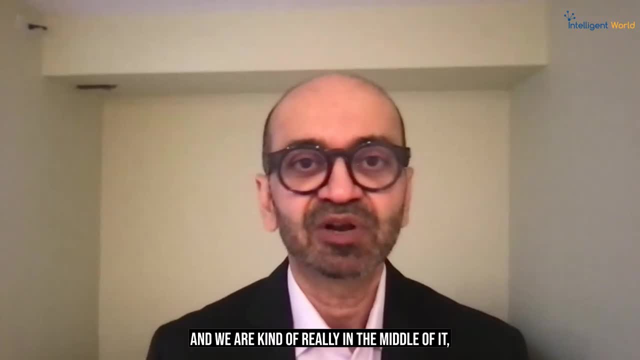 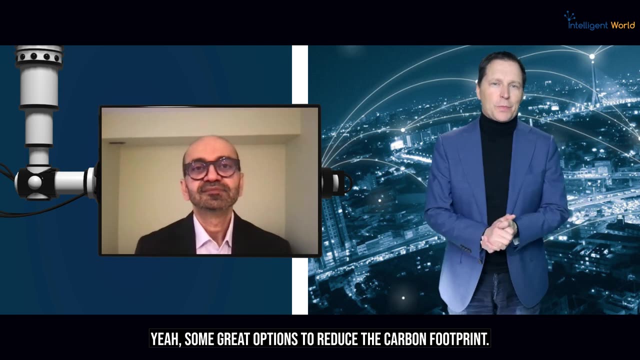 and cloud will play a big role And we are, kind of you know, really in the middle of it, working with all of our telco customers Some great options to reduce the carbon footprint. You were talking about trends three: 5G monetization. 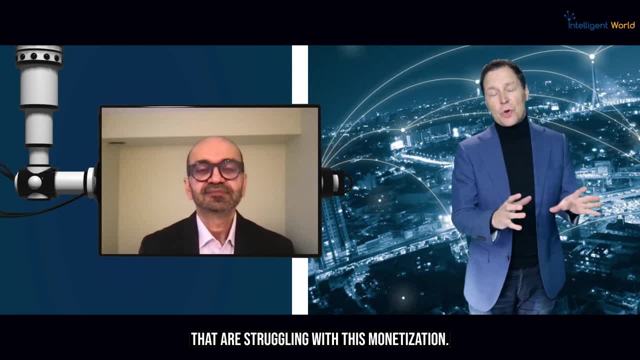 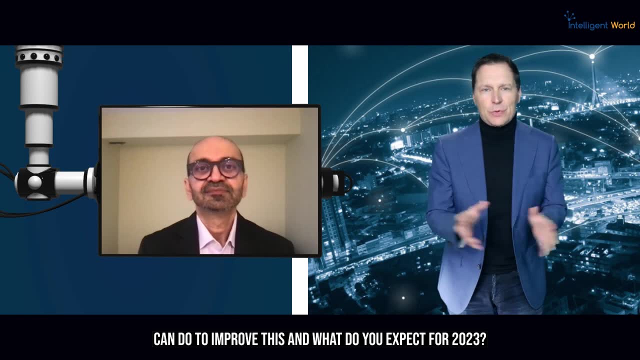 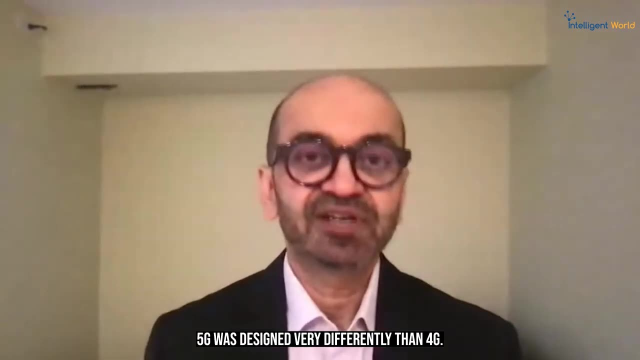 And we see many telecom service providers that are struggling with this monetization. Can you share what telcom service providers can do to improve this And what do you expect for 2023?? Yeah, so the whole premise of 5G. 5G was designed very differently than 4G. 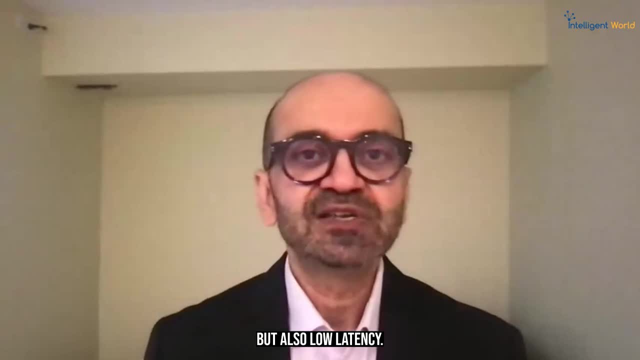 It's not just about higher bandwidth and higher throughput, but also low latency. It's also about a very virtualized network that lends itself to run on the cloud. It's also that also makes it very agile. It's easy, you know, relatively very easy to build new services on top of the network. 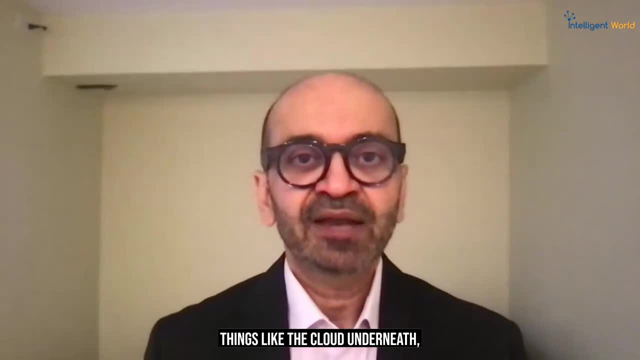 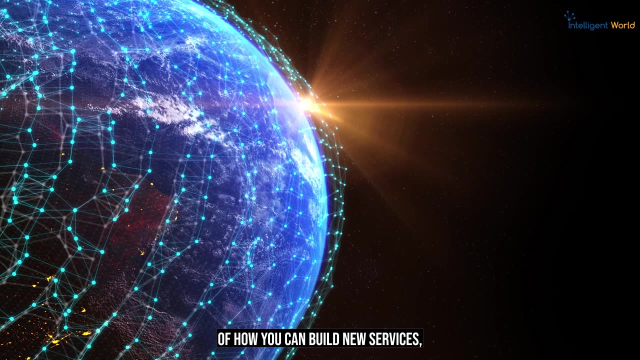 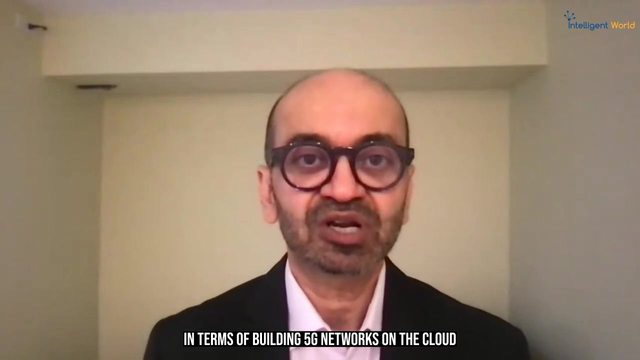 But to make that happen you need things like the cloud underneath. We now have critical mass of 5G networks to start looking at that next layer of how you can build new services, And also we have a lot of traction with customers now in terms of building 5G networks on the cloud. 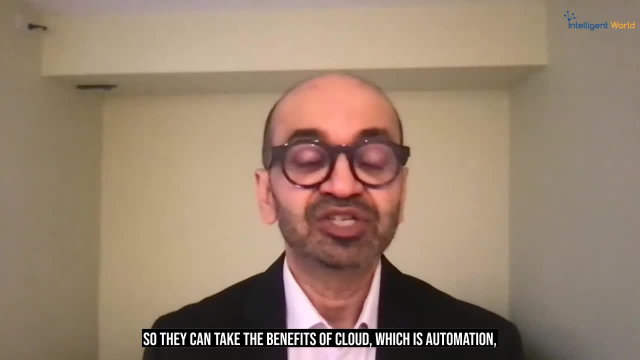 so that they can take the benefits of cloud, which is automation, the agility to build new services, and so on. We have Dish that has built the first fully cloud native network in the US. We have Swisscom, some other companies also. 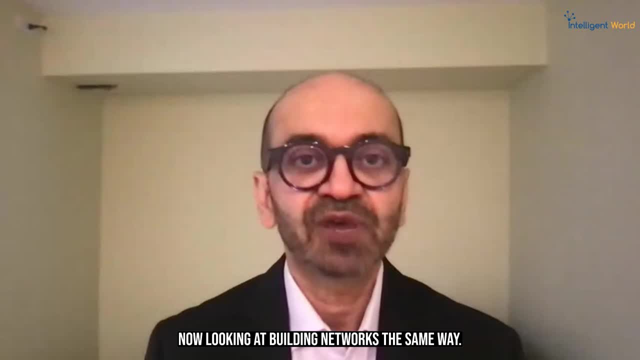 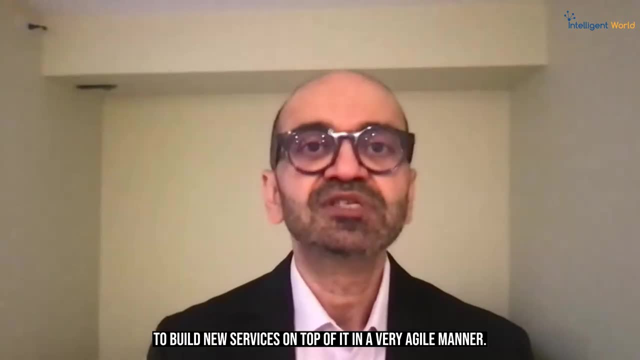 you know several of our customers now looking at building networks the same way. So once we have that in place now, you can get to the next level of really starting to build new services on top of it in a very agile manner. So we recently announced Mobi. 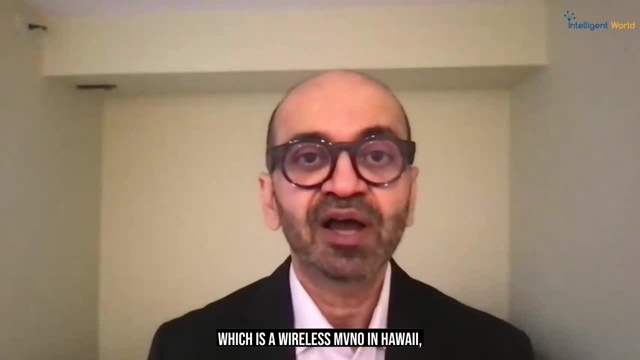 which is a wireless MVNO in Hawaii using Working Group 2's core, running on AWS. Now this is an MVNO leveraging T-Mobile's network, but they've built this using on AWS, So what that has given them is the ability to just use APIs. 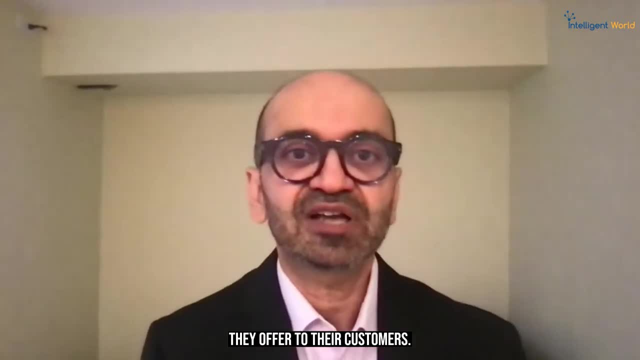 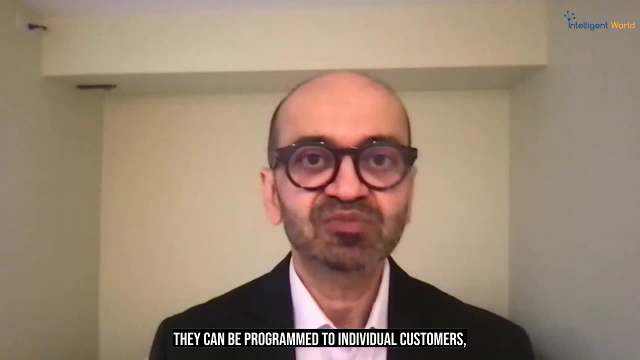 and dynamically configure the services they offer to their customers. Now, these can, because it's dynamic and it's just done with easy API calls. they can be programmed to individual customers- individual SIMs depending upon what they need- and can be personalized. 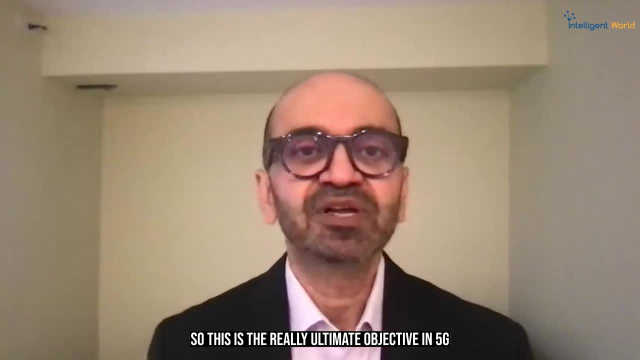 So this is the really ultimate objective in 5G is to be able to do these things dynamically, And we are seeing evidence of that Now. so 5G being built, having critical mass of 5G and the devices that go with it. 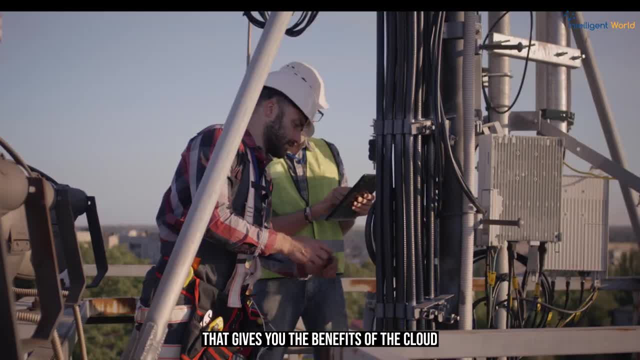 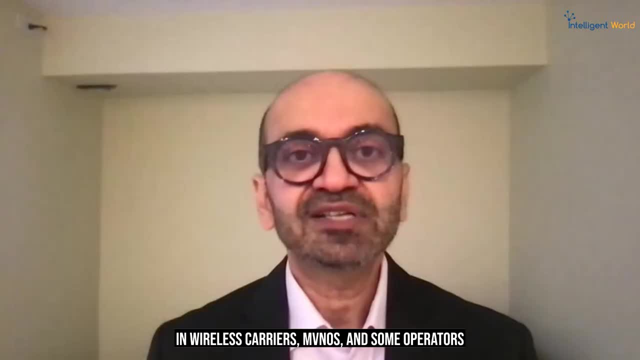 Secondly, starting to use the cloud underneath. that gives you the benefits of the cloud in terms of automation, agility And, lastly, some actual proof points in wireless carriers, MVNOs and some operators starting to experiment and really put this into practice.